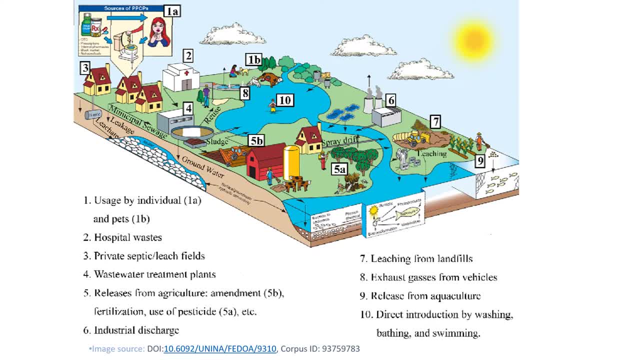 These compounds are produced by a hospital waste, private septic fields, wastewater treatment plants, agricultural land due to use of pesticides, industrial discharge and exhaust gases from vehicles, etc. What are these xenobiotics compounds? So, basically, these are main made compounds like 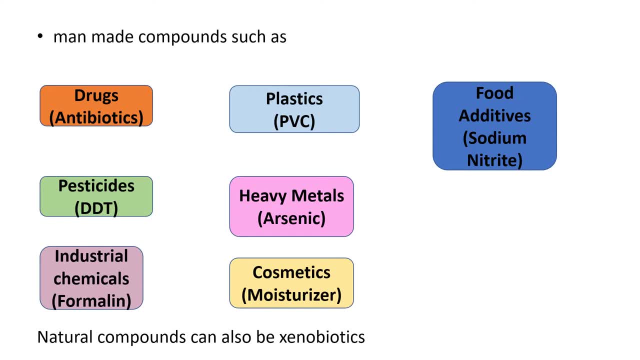 drugs such as antibiotics, pesticides like DDT, industrial product like formalin, plastic like PVC, which is polyvinyl chloride, heavy metals like arsenic, cosmetics such as moisturizer, food additives like sodium nitride. Natural compounds can also be a xenobiotics. 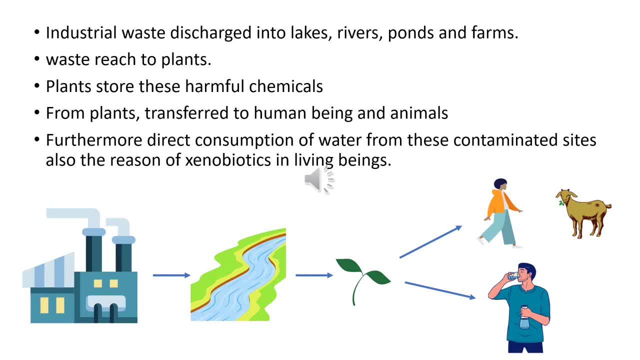 Let's see an example how xenobiotics enters in the body First. industrial waste discharge into lakes, rivers, ponds or farms. From there these chemicals reach to plants grown near by farms and fields. Plants store these harmful chemicals When human being and animals consume these crops or plants. 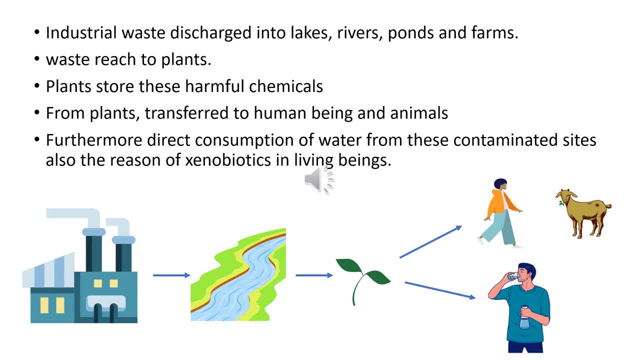 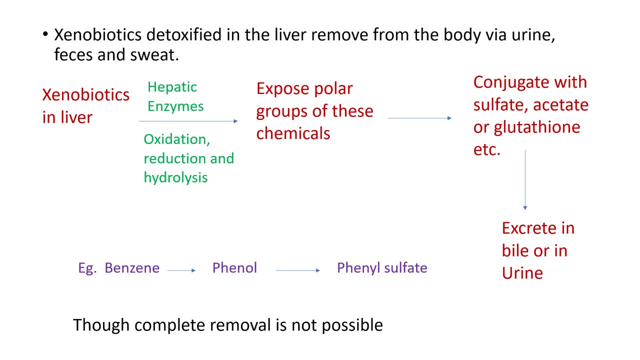 these chemicals reach into their body. Furthermore, direct consumption of water from these contaminated sites also the reason of xenobiotics in living beings Body try to detoxify these harmful chemicals and the process takes place in the liver. Liver enzymes or hepatic enzymes, oxidize, reduced or hydrolyze these chemical compounds. 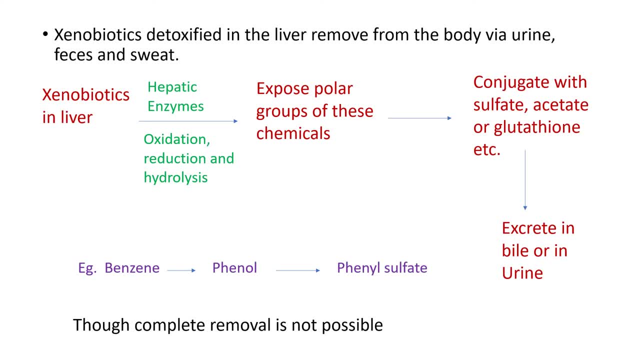 and expose their polar groups. These polar groups conjugate with sulfate, acetate or glutathione present in the liver and finally they take exit from the body via bile On bile, sweat or urine. For example, benzene oxidation form phenol, then phenol reacts. 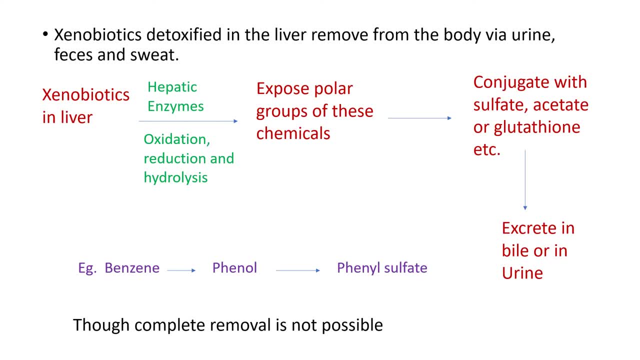 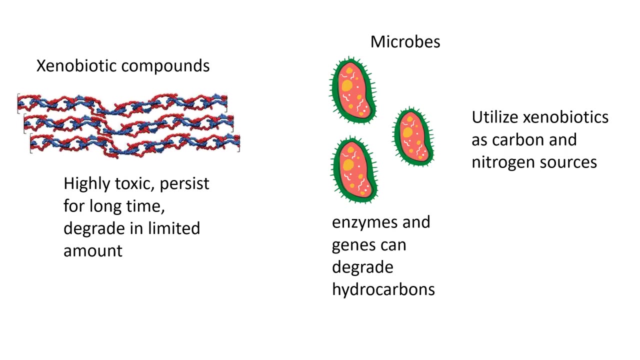 with sulfate present in the liver and form phenol sulfate, which excrete via urine, bile or sweat. Though complete removal of all xenobiotics from body is not possible, Some xenobiotics, such as polycyclic aromatic hydrocarbons, are highly toxic, persist for 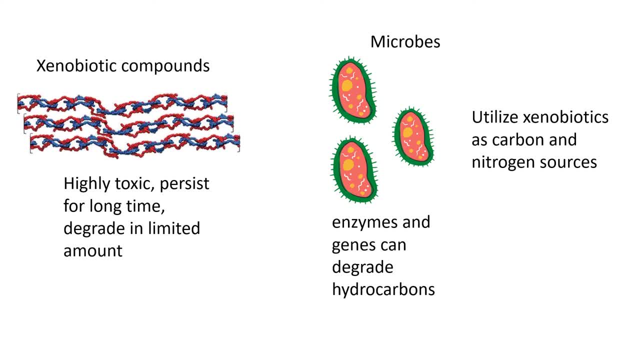 long time in the environment and degrade in limited amount. Microbes which survive in harsh environment have a potential to degrade such toxic and harmful compounds. Microorganisms have such genes and enzymes which catabolize xenobiotics. They utilize xenobiotic contaminants.